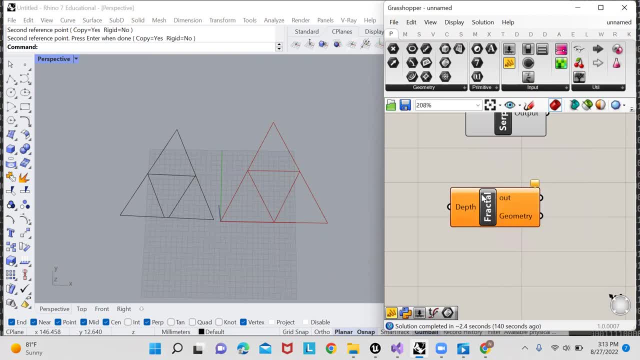 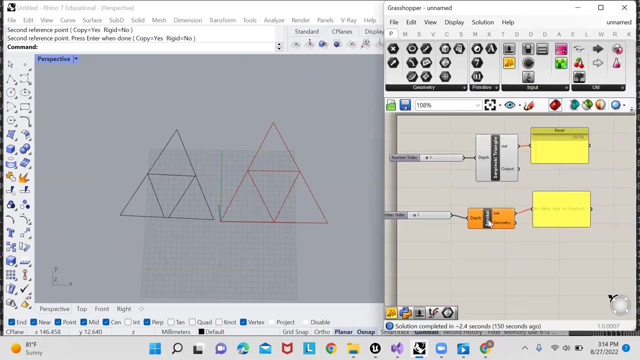 And I could even name this to fractal. And now we're ready to start scripting, After we hook up our depth and our panel, just so that we can send ourselves messages by using print statements. Okay, let's write some code. 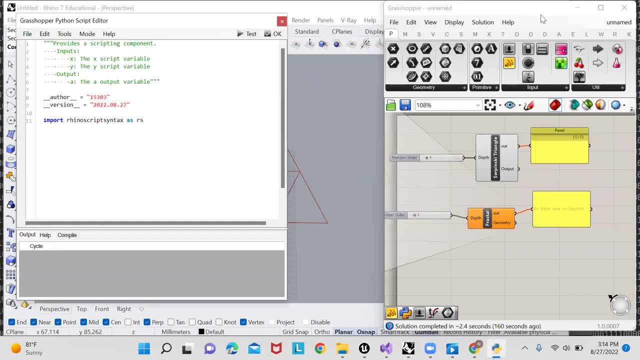 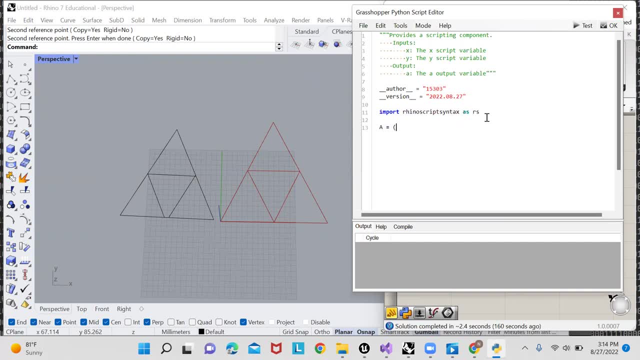 If I open this editor, I can start making the initial triangular polyline just by creating three points. Points are simply tuples, which is a list of values surrounded by parentheses. So the first point of the triangle will be at the origin. The second point will be at 50,, 100,. 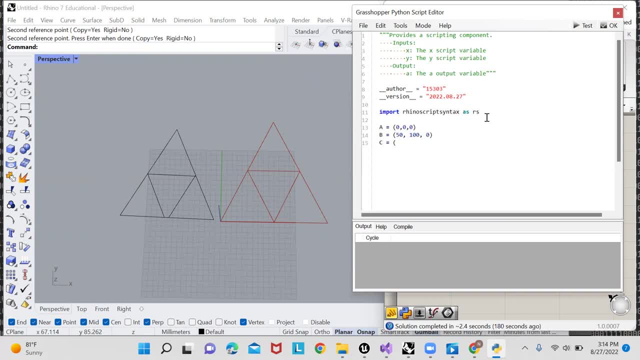 0, and point C will be at 100, 0, 0.. And now to create a list of triangles and initialize it with our very first triangle. I'm just going to type out triangles, equals, and then a list, And inside that list we'll have to create our first triangular polyline by typing out rsaddpolyline. 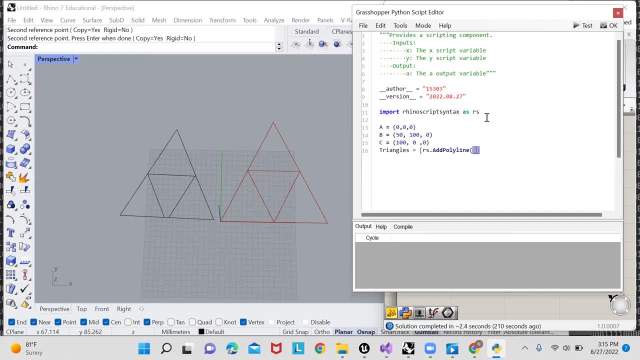 And if I just throw a list of points into this polyline function, it'll create a polyline. So I'll just type in A, B, C and then back around to A to close off our polyline, And just to verify that this is working so far. 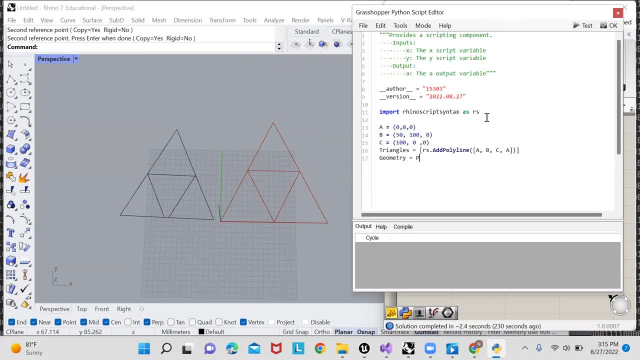 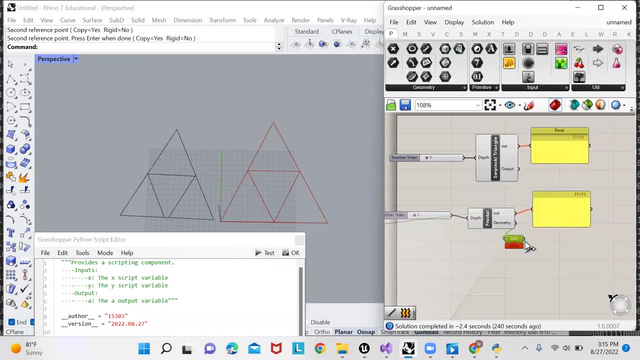 I'm going to say geometry equals triangles, And let's test our code. You can see everything ran well because there's no red. And if I hook up a line to the output of geometry? well, that didn't work. I could hook up a polyline to the 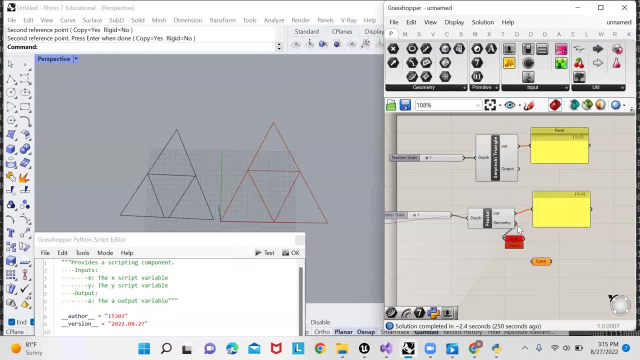 or a curve. I suppose A polyline falls under the category curve. You can see that that worked And if I hover over here you can see one value inherited from one source: polyline curve. The reason it didn't work for a line is because a line must be one straight line. 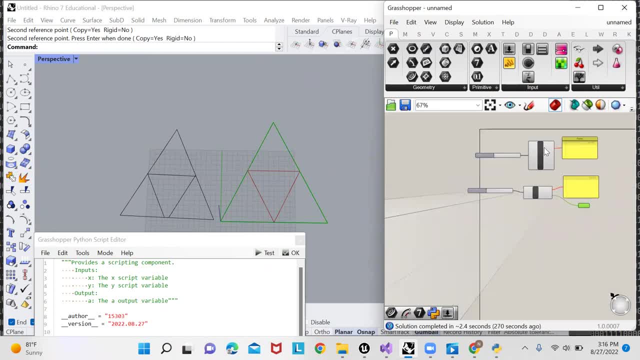 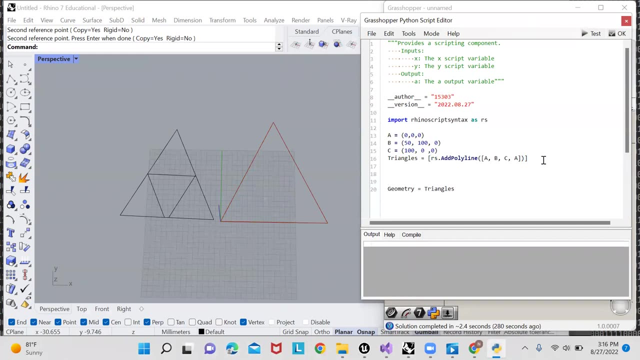 All right. So, since that worked and we now have our triangle, well, let's disable- or, yeah, let's disable- this previous program so we can see what we're working with here And now it's time to write our function, So we're going to want to repeat all of these steps as many times as there is depth. 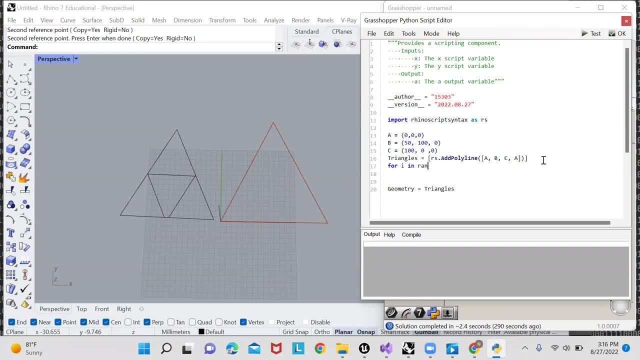 So we'll say: for i in range depth, we will repeat this process of creating a new list of triangles. So we'll say new triangles and we'll leave it as an empty list for now, And then for each triangle in the old list of triangles. 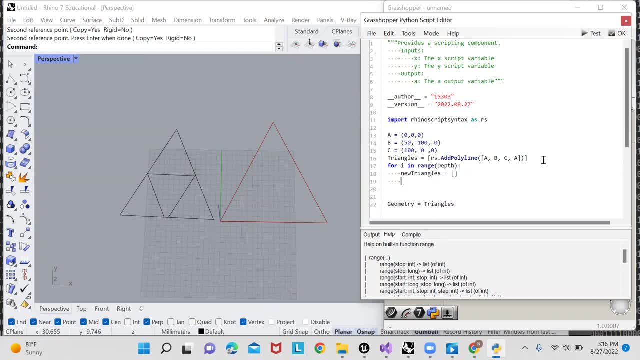 we'll have to make three new triangles and toss it into this list of new triangles. So we'll say, for triangle in triangles and to find these three new triangles that we're going to toss into the new triangles list, all we need to do is find all of the centers that we're scaling around and scale by them. 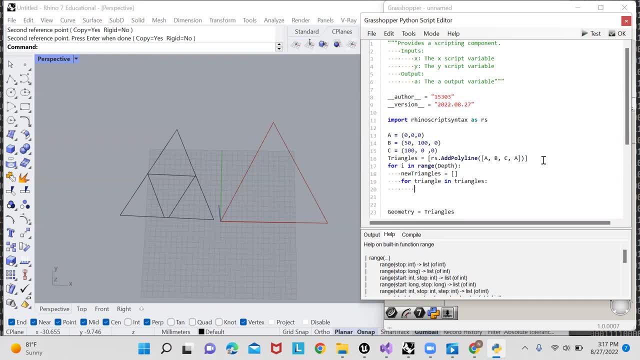 So to find these centers that we're scaling around, we just need to find the points of the polyline which are rspolyline vertices, And if I just pass in my triangle, it'll return a list of points which are the vertices. 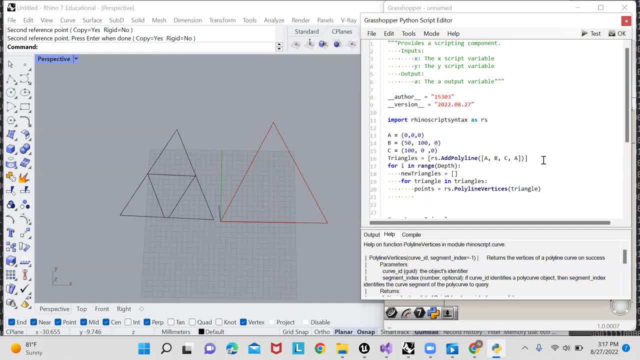 So now, for each one of these points, we're going to want to scale the triangle around that center point and then put it into this list of new triangles. So I'll say new, or actually, for i in range three. So for each corner of the triangle, 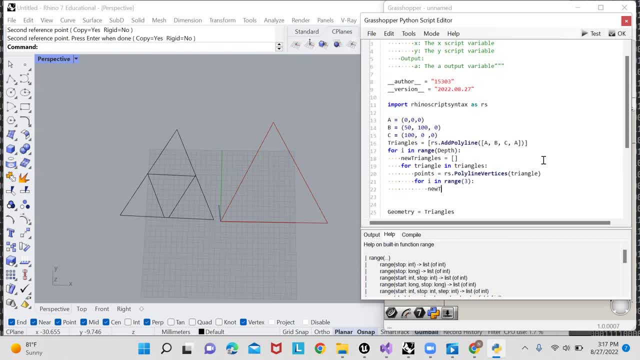 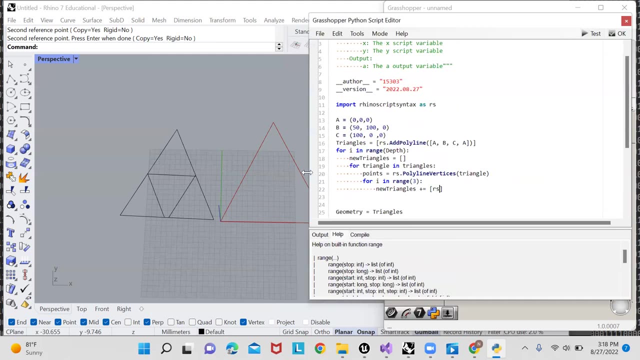 we're going to want to say new triangles plus equals, And then we're just going to merge it with this new list containing the new triangle, And we can create this new triangle by typing out rsscaleobject. And if you're wondering how this scale object function works, 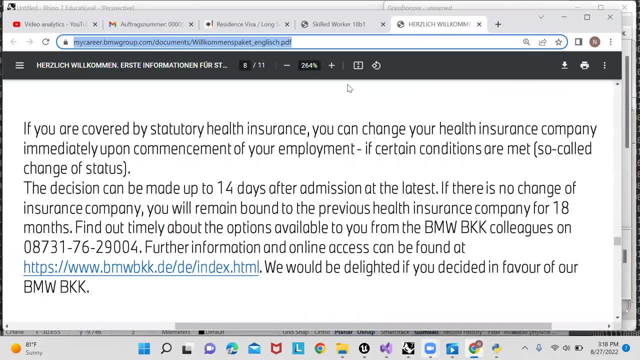 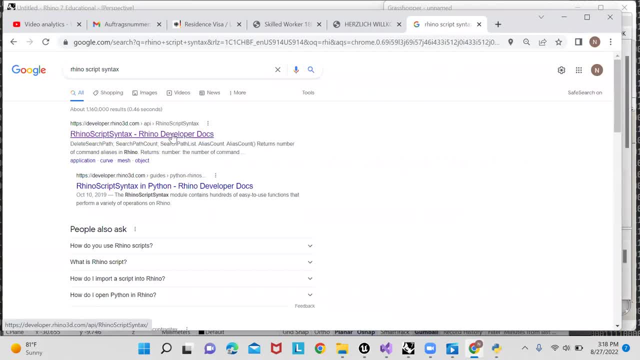 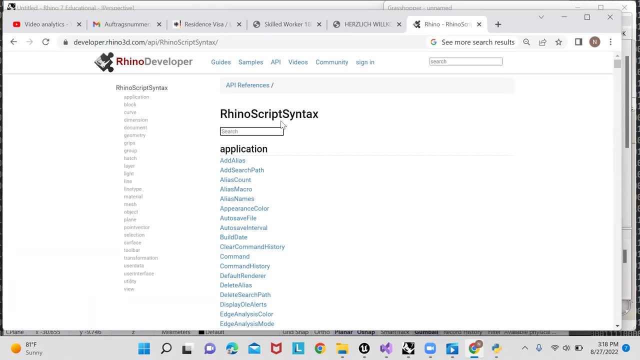 I should mention that you can just open up a Chrome tab and look up Rhino script syntax and Rhino developer docs. this first tab is the one and you can look under all these categories or search up any function to find the specifics. So if I want to know how scale object works, 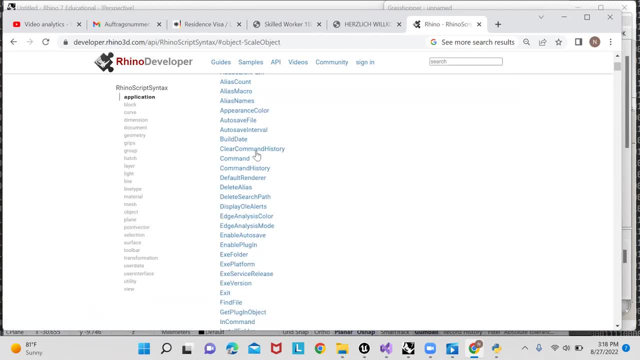 I'll just type in scale object right here and it'll bring up the parameters, the return values of the function, and it'll even give me a nice little example And, as you can see, we have the object, the point we're scaling around. 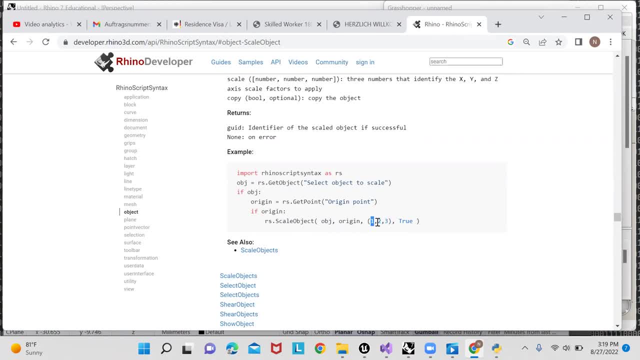 the scale factor. we're actually three factors. This is a scale factor in the x dimension, scale factor in the y dimension, scale factor in the z dimension. and true meaning. we want to copy the curve and not scale it itself. We want to make a replica of it that's scaled. 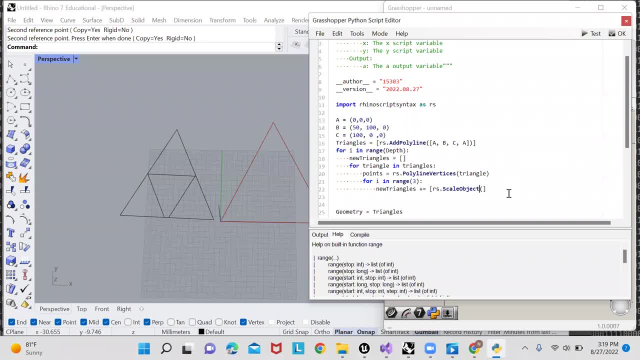 Okay, So let's return back now that we know how rsscaleobject works. And so what are we scaling The triangle? What are we scaling around This point, which is points of i, because points is the list of all points. 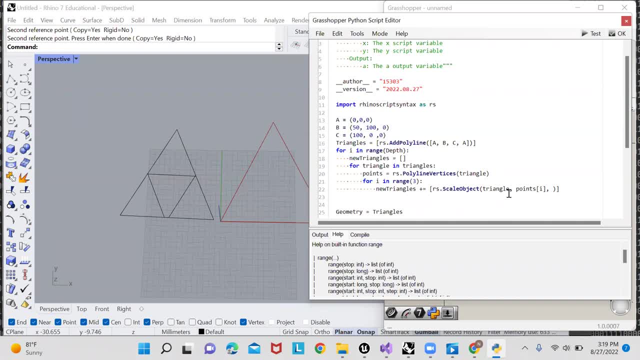 and i is which point we're using. What are the scale factors? Well, 50%, So 0.5,, 0.5, 0.5.. And then do we want to copy it? Yes, So I'll just say true. 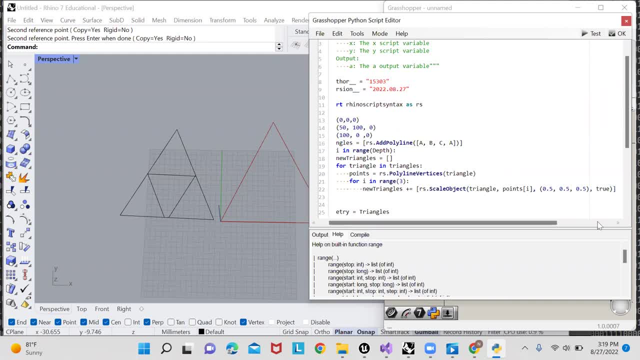 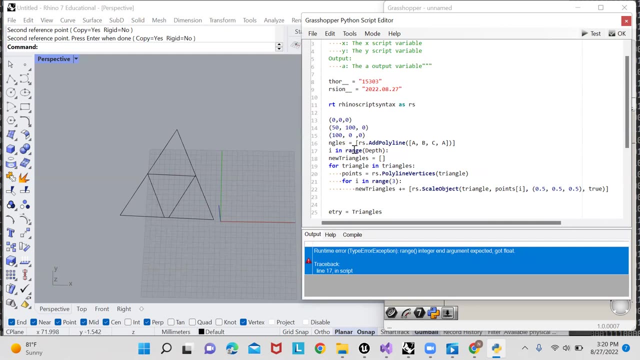 And I think I have one too many parentheses here. And now, if I test, you can see on line 17,. range integer argument expected got float, So let's go to line 17.. So it's expecting an integer here, but I've inputted a float. 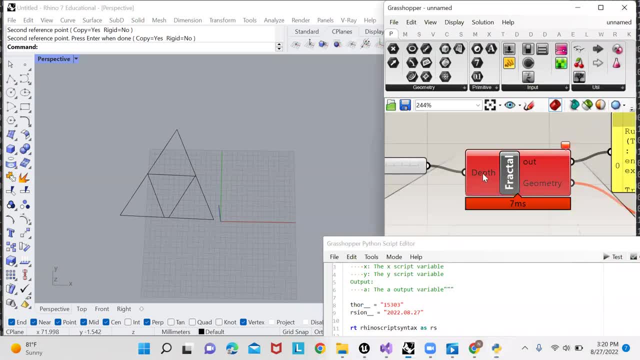 So let's go check and see what the type of this depth is. So I'm going to set the type hint, because it should be integer, And I set it to integer. I test it Now. I got a new error, So it was interpreting this as a float.